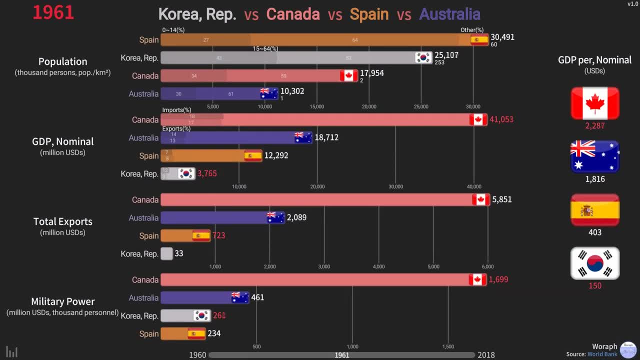 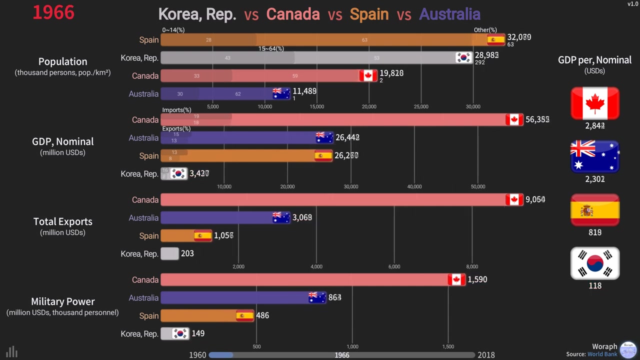 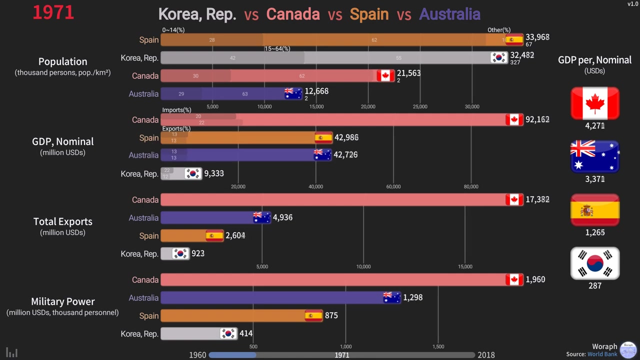 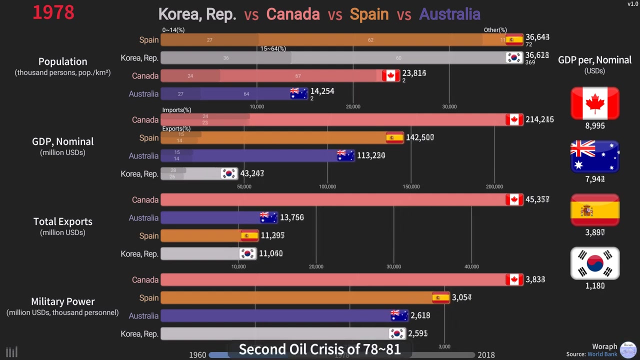 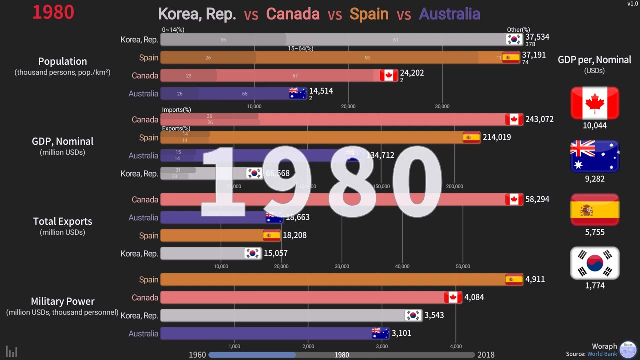 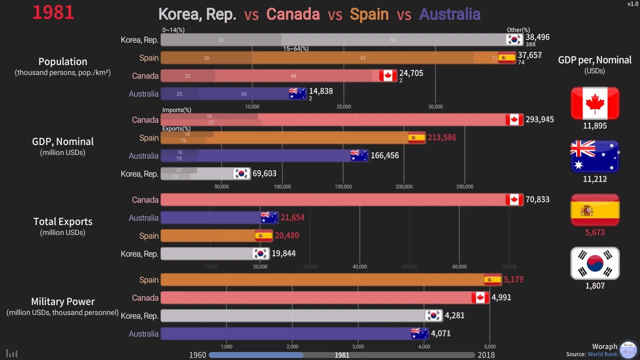 Thank you for watching the video. Please subscribe to the channel and press the bell to receive notifications when I upload a new video. Please subscribe to the channel and press the bell to receive notifications when I upload a new video. Please subscribe to the channel and press the bell to receive notifications when I upload a new video. 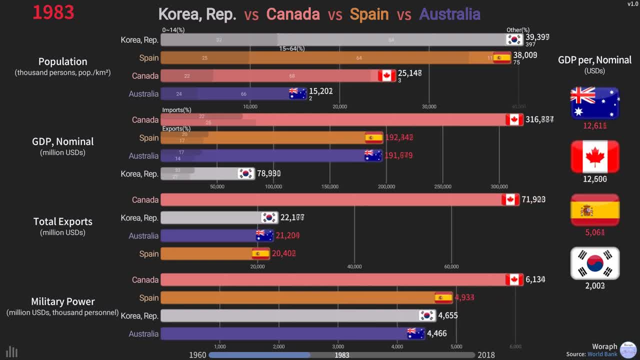 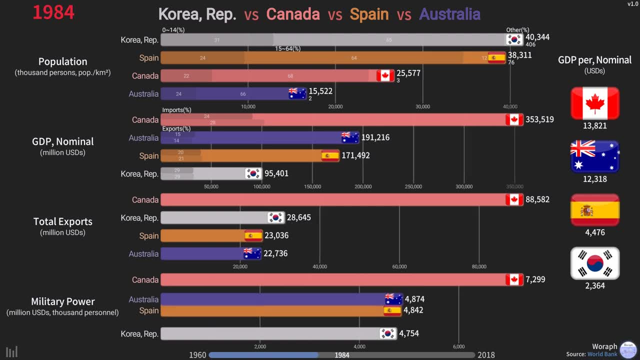 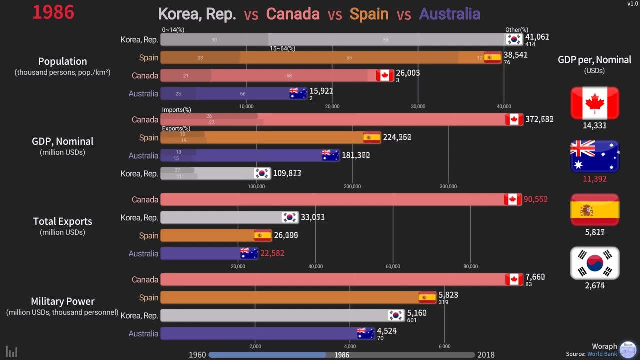 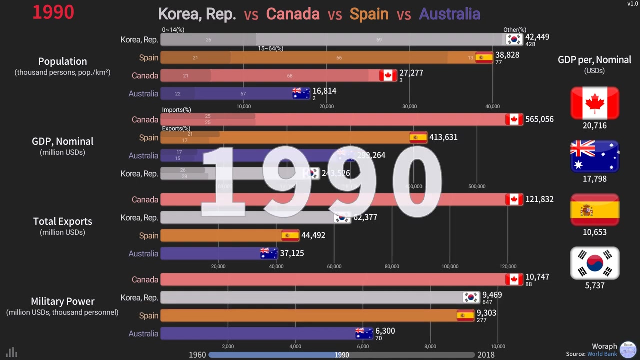 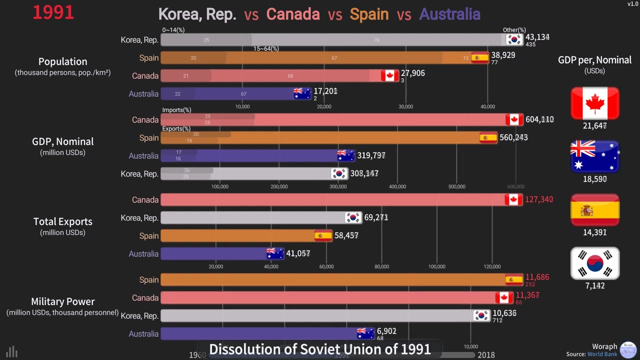 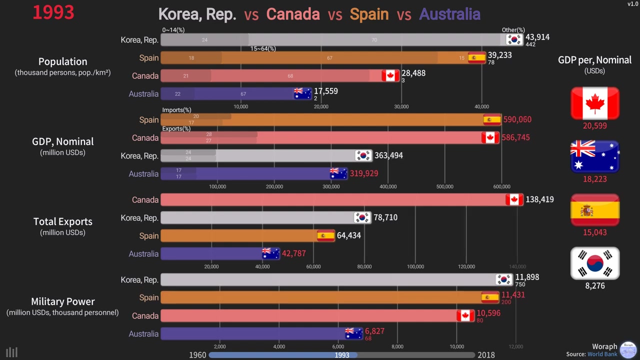 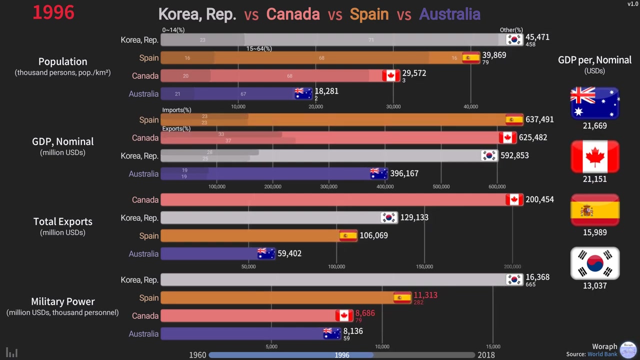 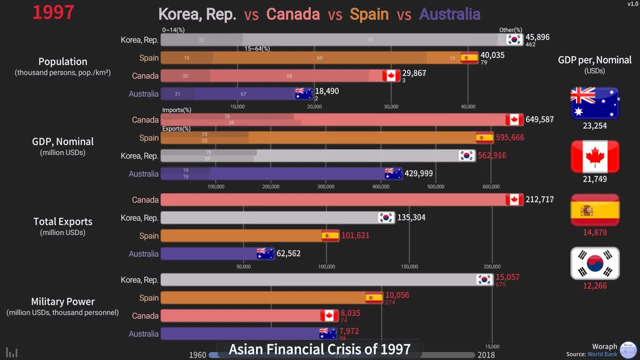 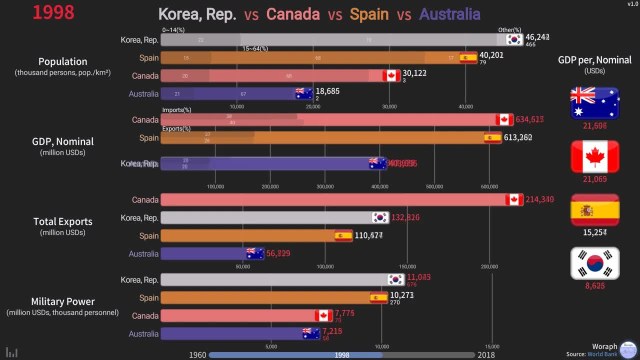 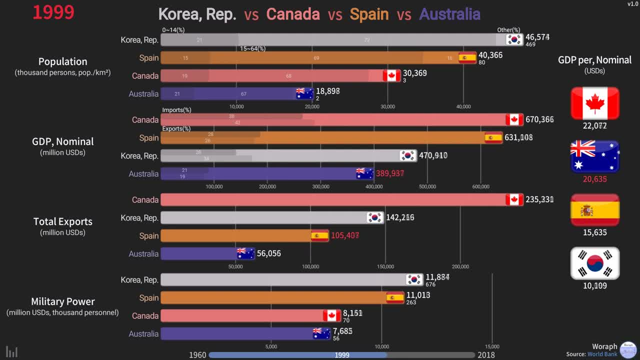 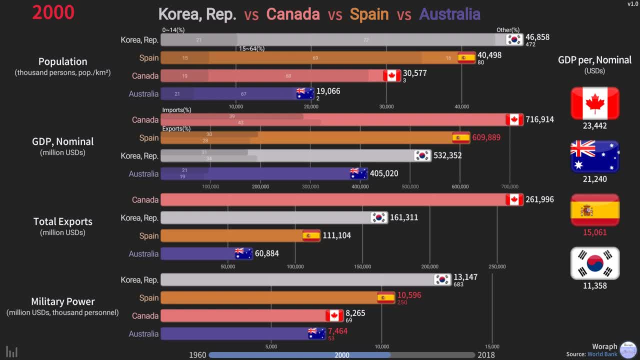